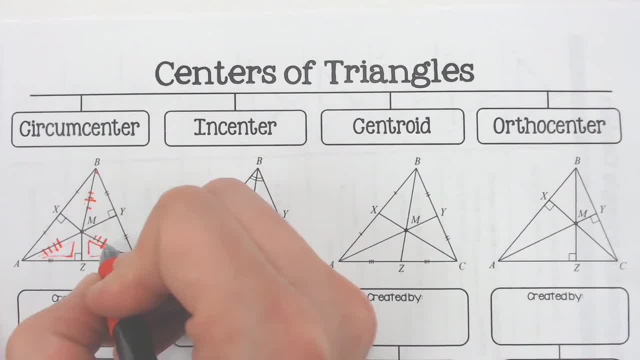 one, two, three, four, and one, two, three, four, because we've already used so many hash marks. We've already used one, two and three up, So I had to use the four, which is almost absurd. 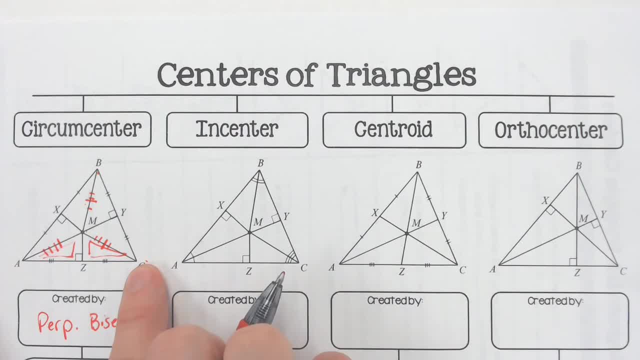 So perpendicular bisectors and the parts that are equal are from the center to the corners of the angle. So you cut the sides in half with a 90 degree angle and it's from the center to the Trans, to the corners that are congruent. The in-center, however, is created by the angle bisectors. 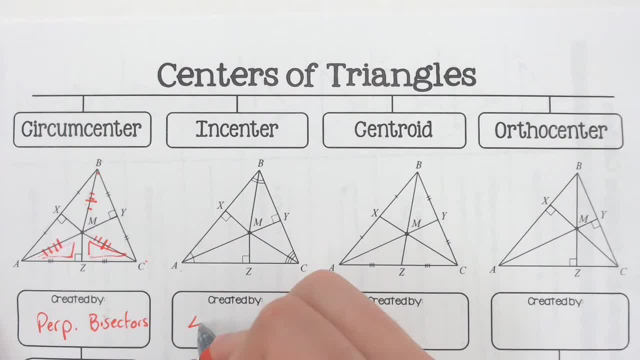 or you cut the corners in half, So you got to bisect each corners. It is created by the angle bisector And the part that's congruent is here: from the side to the center, from the side to the center and from the side to the center, The triangles that are congruent are from: 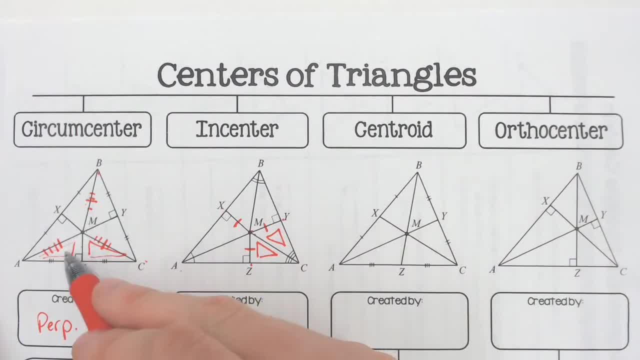 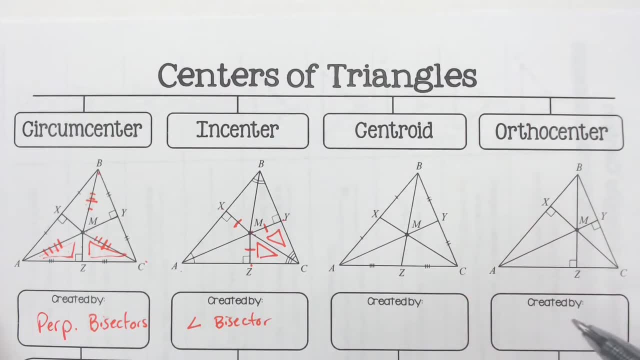 the corners as well, not from the sides, And the centroid is having zero triangles that are congruent. It is a little more recognizable because there's no 90 degree angles in it either. Notice how the other two had 90 degree angles. 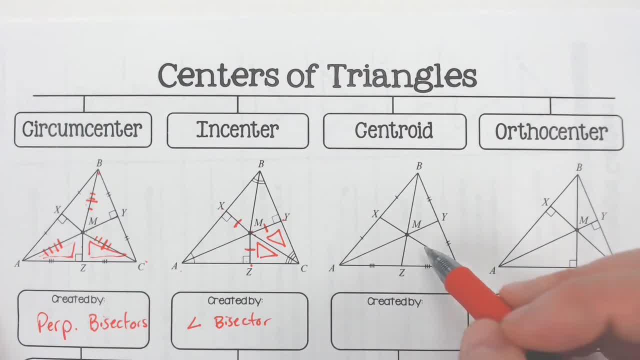 This one does not. So the centroid is found by just taking the sides, and you cut the corners as well, from the sides to the center and from the sides to the center. Notice how the other two had 90 degree angles. This one does not. So the centroid is found by just taking the sides and 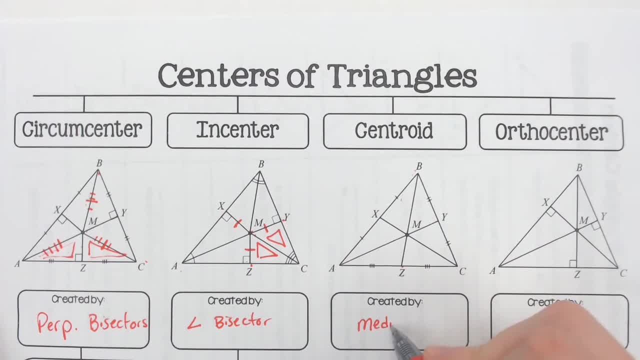 going straight up. It is created by the medians of the triangle, which is going from the midpoint straight to the other angle- Not straight up but straight to the other angle. And it does create that special relationship where, if this is 20, that part would be 10.. It is half, Two times the 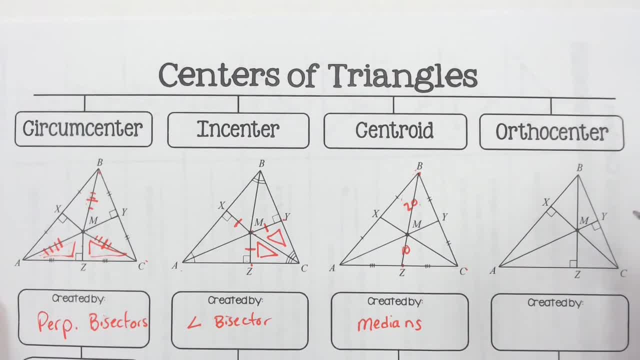 short part equals the longer part. New one for most people is probably going to be the ortho center. Ortho center is kind of it's the weird uncle nobody talks about. Ortho center doesn't have a lot going on. It's kind of a weird uncle nobody talks about. Ortho center doesn't have a. 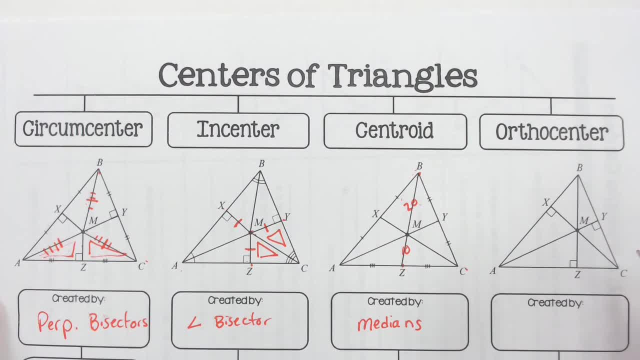 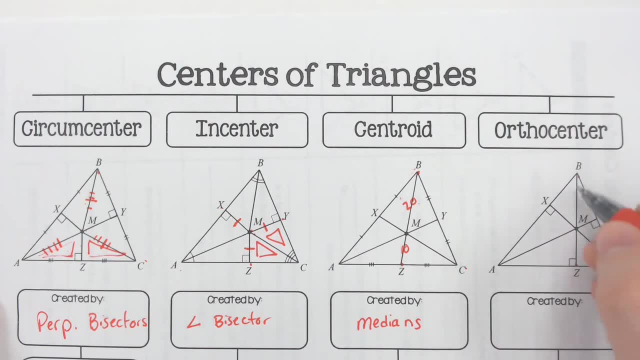 lot going on. There's not much that it actually does. It is the height of the triangle, which is kind of neat, because if we were going straight here, that would be how tall this triangle is. So it's found by taking the heights. It's the intersections of all the heights of the triangle. 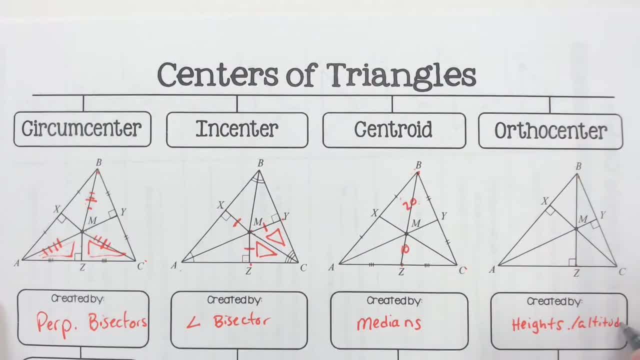 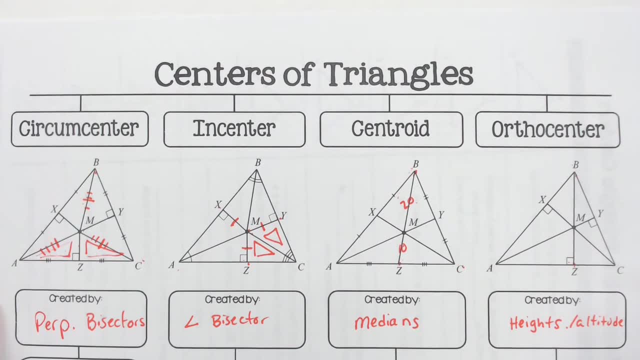 which is also called the altitude. I like height Of the triangle. It does have 90 degree angles because in order to go straight up, you got to go straight up, being perpendicular to the bottom. So it's kind of neat because if we were going straight here, that would be how tall this. 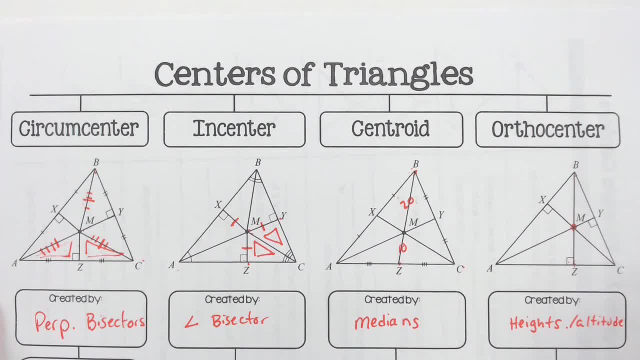 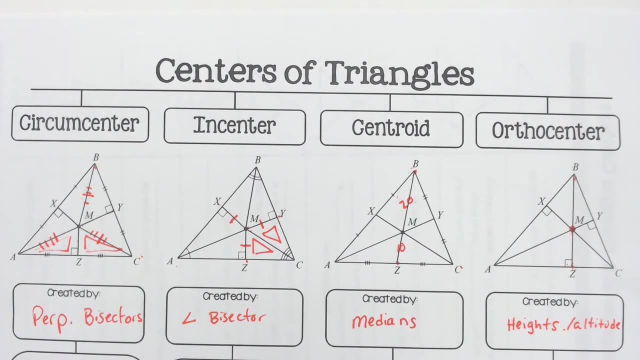 triangle is, And that is all that really characterizes the ortho center. There's no congruent triangles at all, There's no relationship between the short and longer side at all, And it's just where they intersect from the heights or altitudes. Okay, So we're going to take a few. 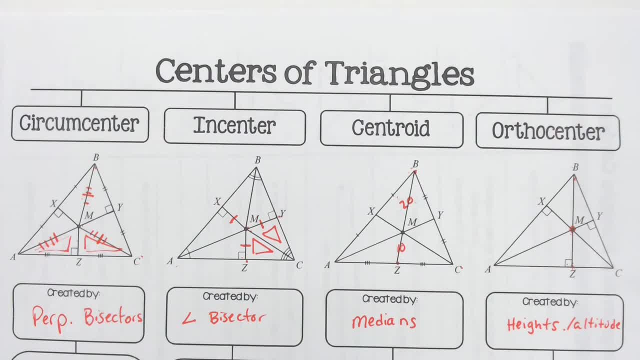 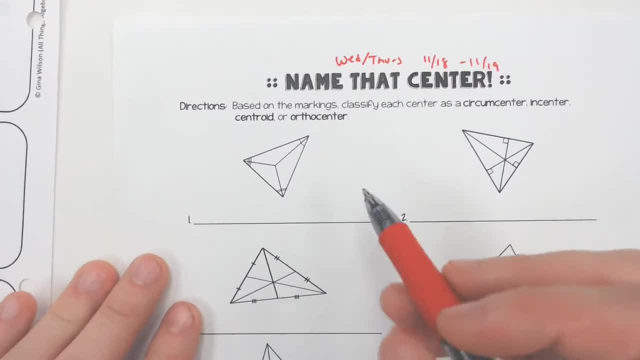 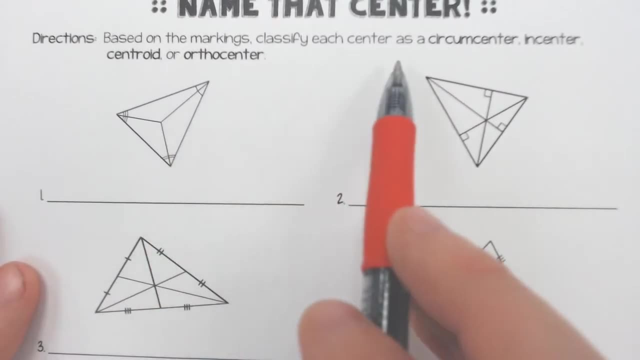 practice problems and we're going to see which, if we can identify which is which. Okay, So here are some practice problems. We have to identify what's happening. And if we're going to identify what's happening, then we're going to be able to name that center. So we're going to call it the. 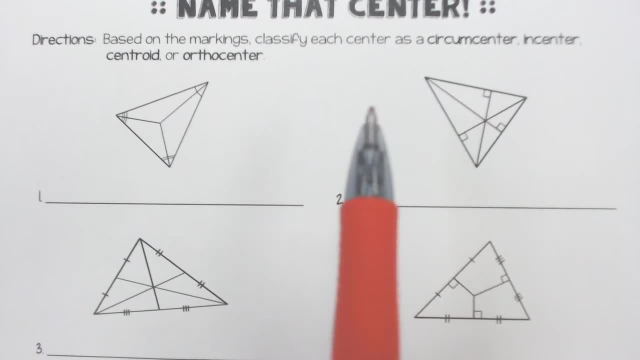 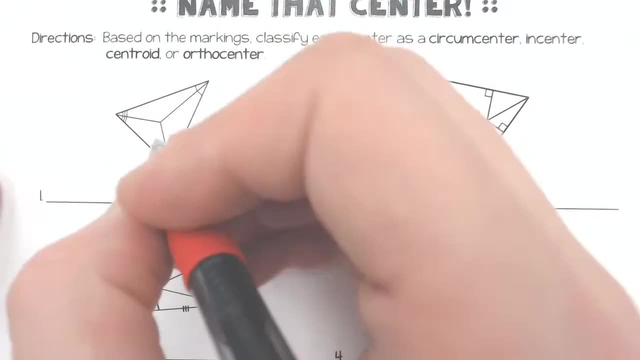 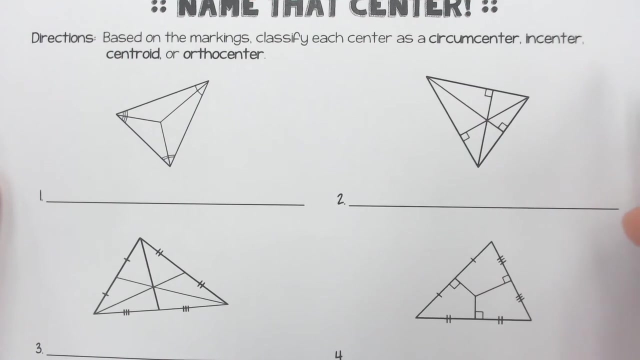 circumcenter, the centroid or the in-center. Let's figure out which one's which. Let's fix the zoom. There we go, Zoom better. So here it looks like we took the angles and cut them in half, And then we got to figure out which. one cuts the angles in half And the angles are cut in half. 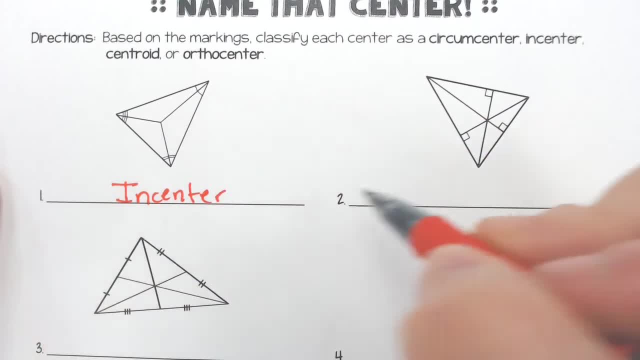 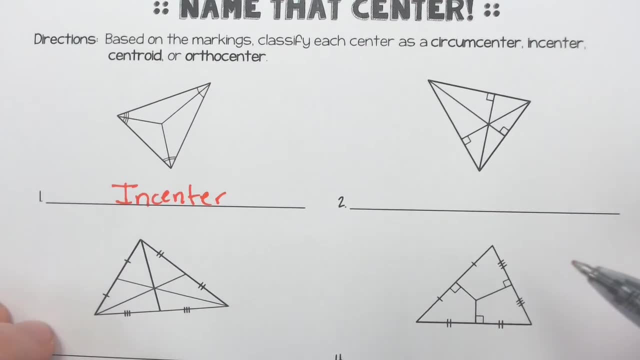 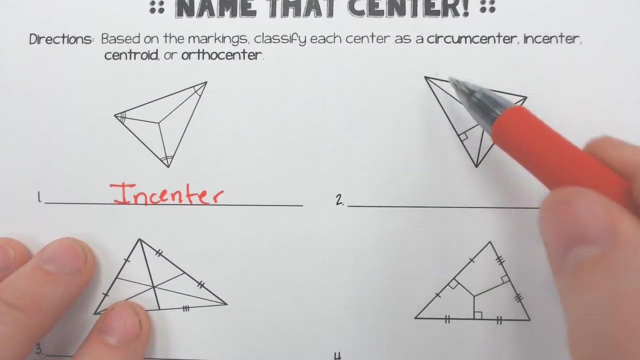 from the in-center. So you'd have to figure out which one cuts the angles in half from the in-center. So go back to your reference guide and figure out which one cuts the angles in half. Here the only thing we're given is that these are 90 degrees and it goes straight up every time. So which one has? 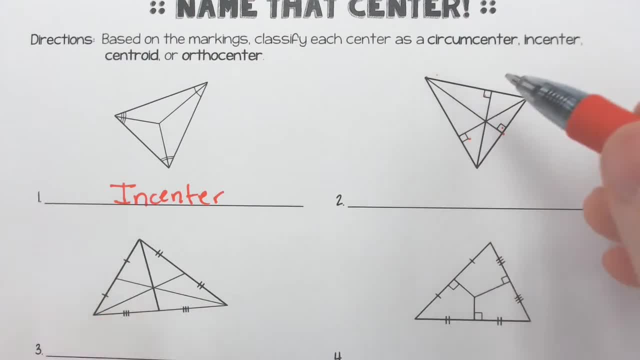 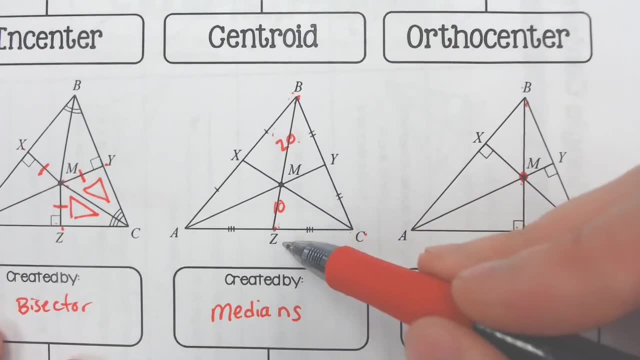 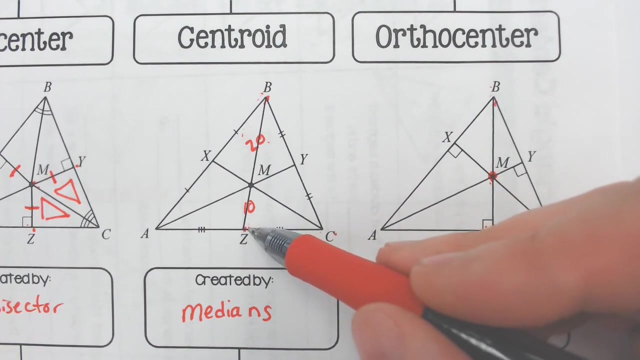 90 degrees here and goes straight to the other side. So there's a few of them that connect the side all the way to the angle straight, And that would either be the centroid or the orthocenter. The orthocenter goes straight with a 90 degree where the centroid doesn't have to. So this one 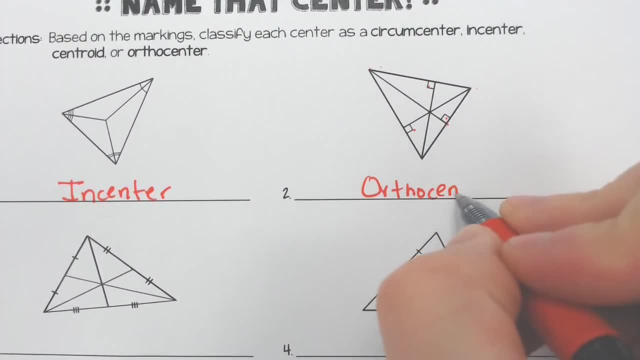 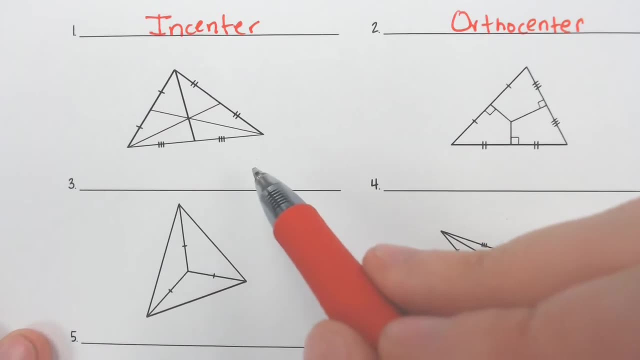 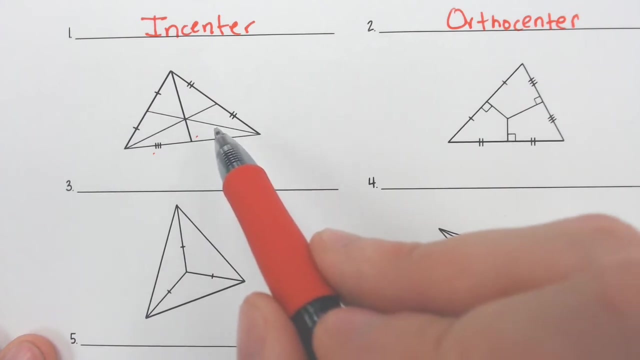 right here is the orthocenter Three. We took the angles, We took the sides, We cut them in half And they're not with a 90 degree angle, So it's not going to be anything with a 90 degree angle. 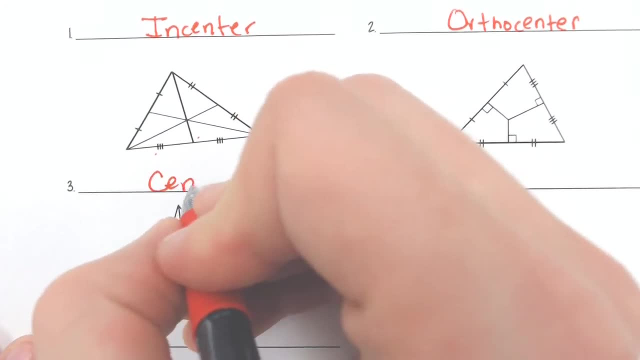 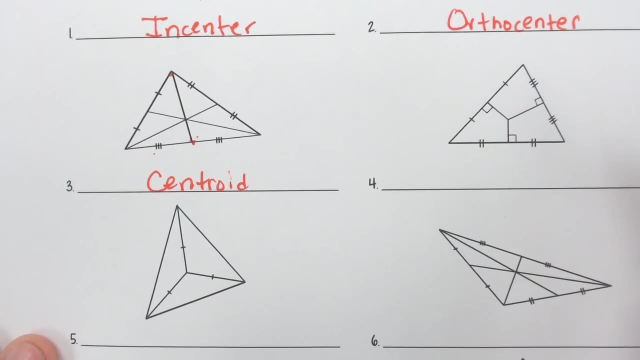 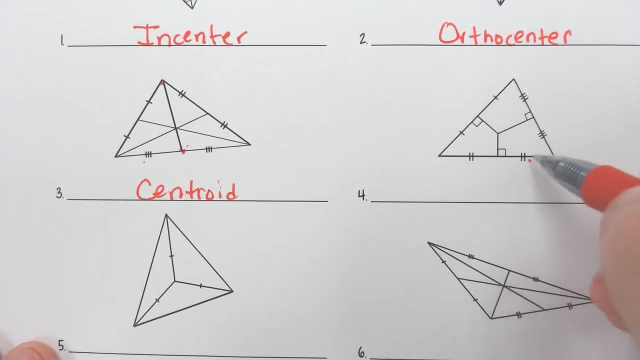 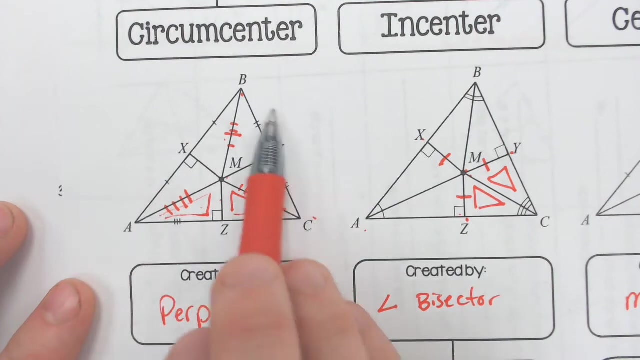 And that means that there's only one possibility. This must be the centroid, because we took the middle and we went straight to the other angle, Number four: Here we bisected the sides, So which one bisects the sides With a 90 degree angle perpendicular bisector is going to be the 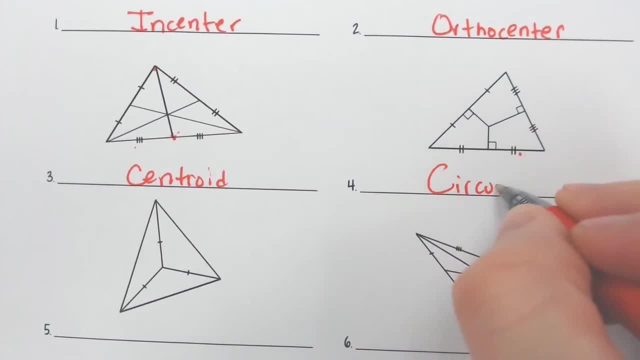 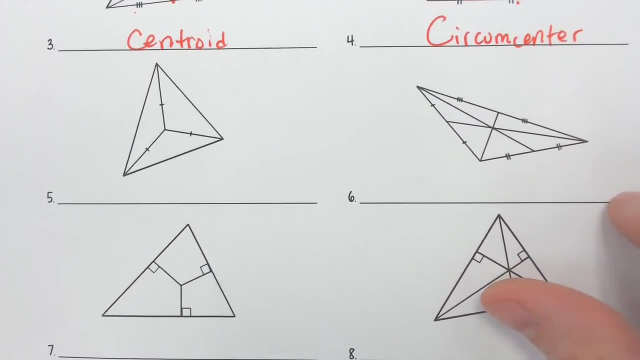 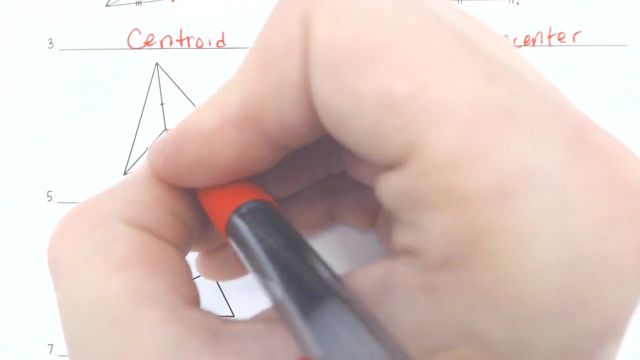 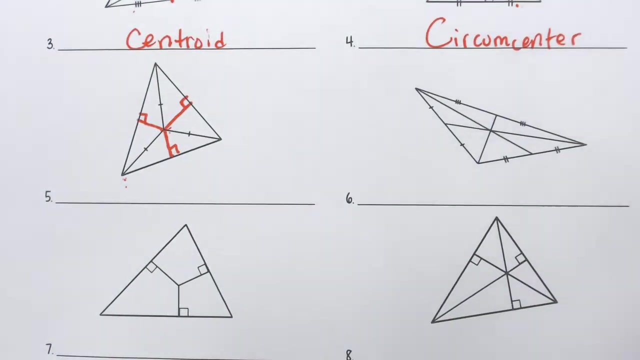 circumcenter, Keeping our triangle triangles right along. Here it looks like we went from the angles straight over and the angles straight over. So what I would suggest when you have problems like this and you might not be sure, draw the line that would make these 90 degrees and then determine whether or not the sides were. 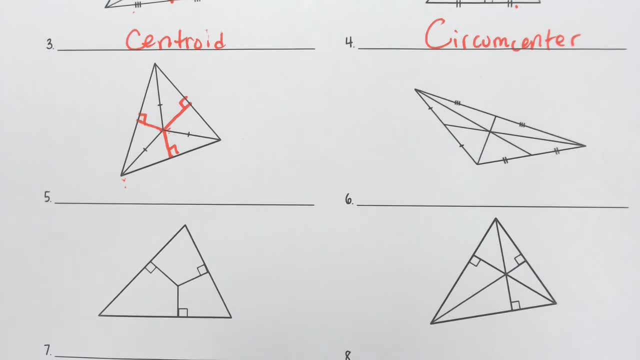 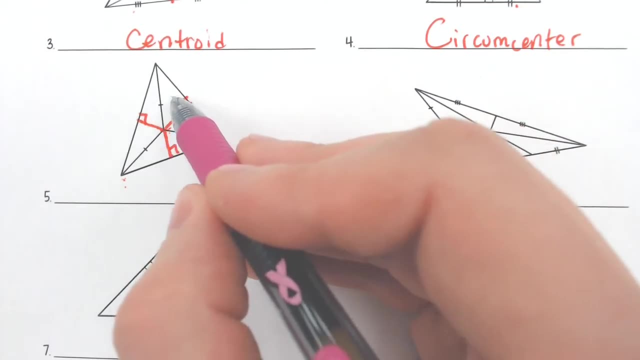 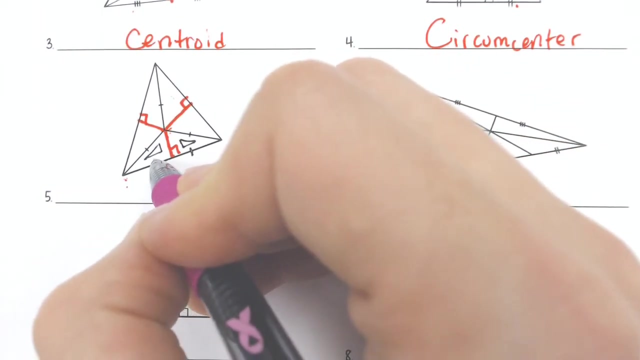 cut in half or the angles were cut in half. So in this case it doesn't look like these two triangles right here and here are really congruent, And it really looks like these are the ones that are congruent, And that means that this side had to have been bisected with a 90 degree angle. 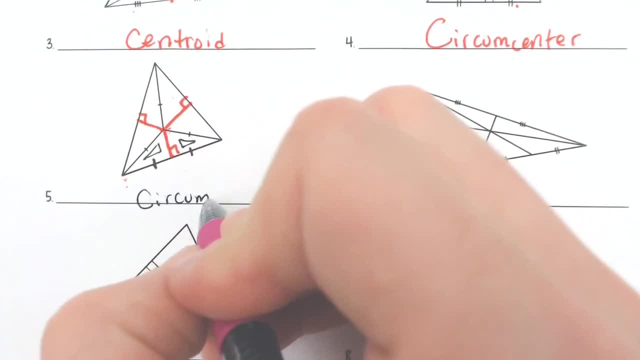 That means that this again is the circumcenter And if we go back to our reference sketch, we're going to see that this is the circumcenter. And if we go back to our reference sketch, we're going to see that this is the circumcenter. And if we go back to our reference, 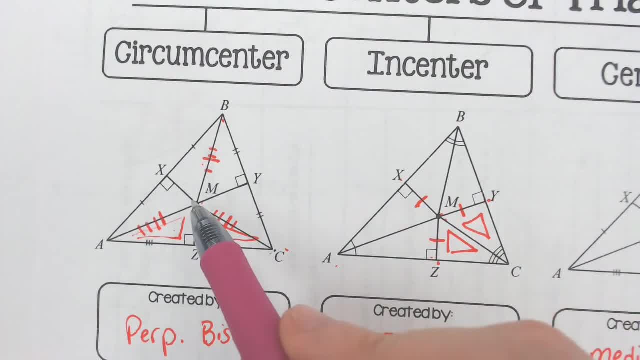 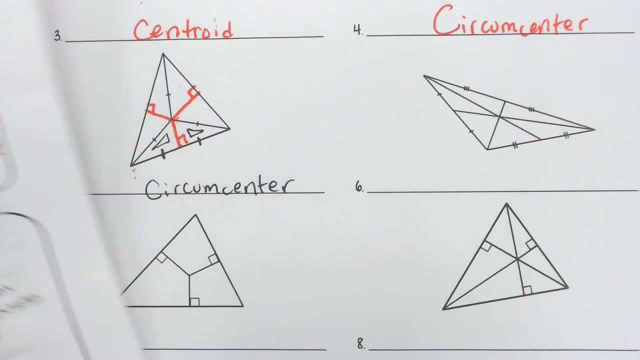 guide. that was what we established with our circumcenter. that from the angle to the circumcenter is congruent. The in-center it's from the side. The side to the in-center is congruent. Excuse me, Number six, It looks exactly like number four or number three did. 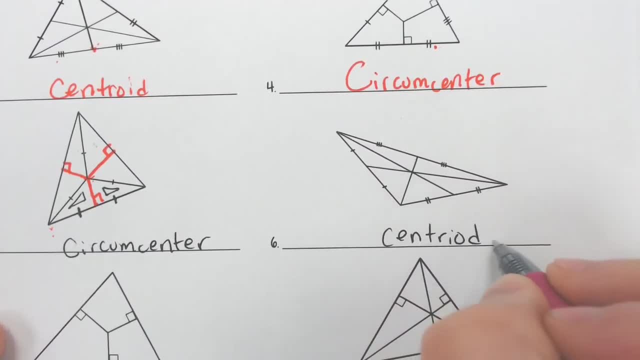 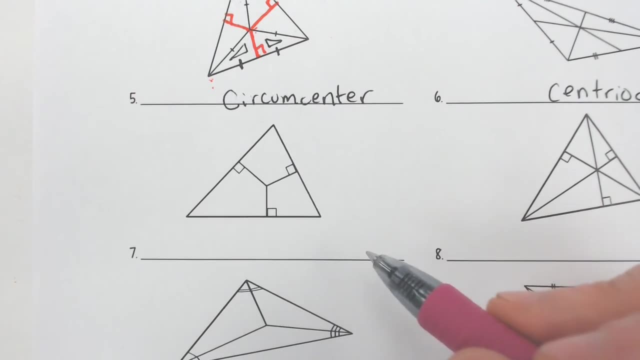 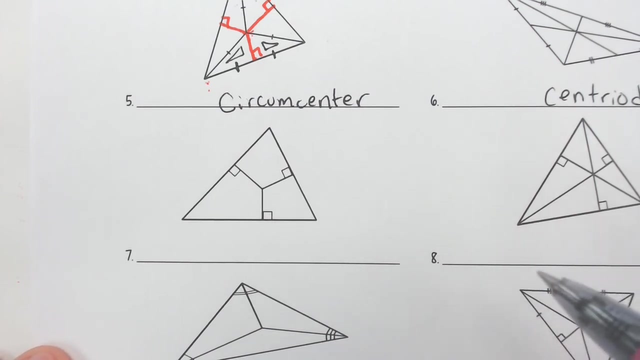 This is the centroid. You found the middle of each one and you went straight to the other angle. What about number seven? Hmm, Number seven doesn't have a lot of information here, And I believe that the problem meant to say that those are congruent. So if these are congruent, this is going to be the in-center, And if I drew 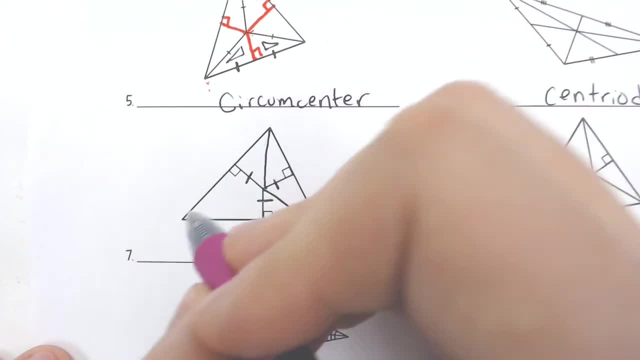 my line straight to the angles. here you can kind of see how these triangles that I'm making from each corner, these triangles, all of these ones coming from the corners here and here, they're going to be equal. This is by far the in-center.